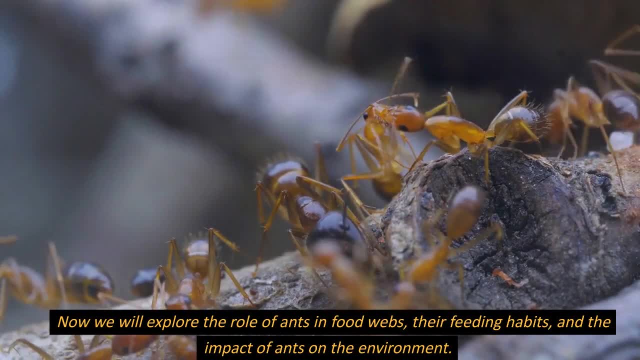 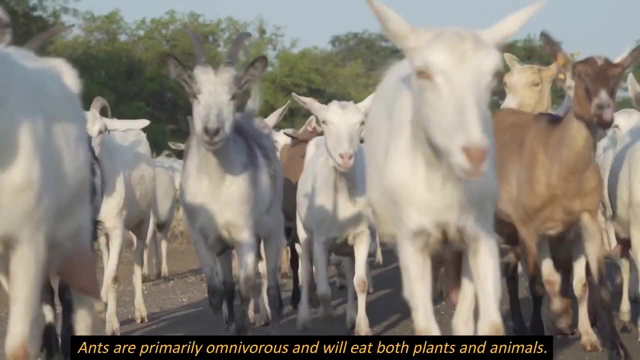 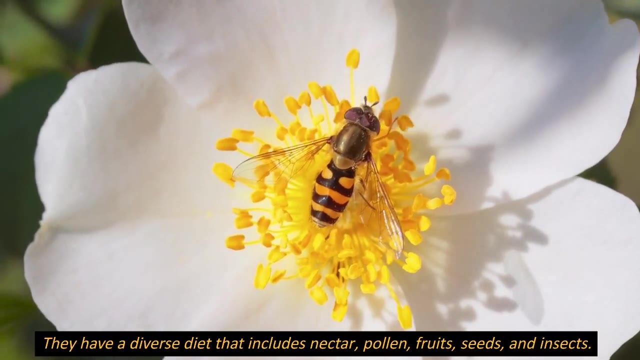 Now we will explore the role of ants in food webs, their feeding habits and the impact of ants on the environment. Ants Feeding Habits. Ants are primarily omnivorous and will eat both plants and animals. They have a diverse diet that includes nectar, pollen, fruits, seeds and insects. 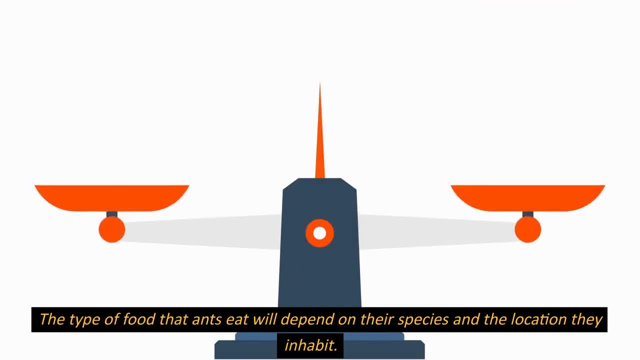 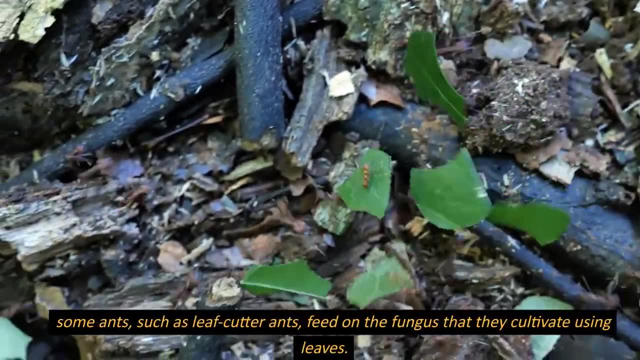 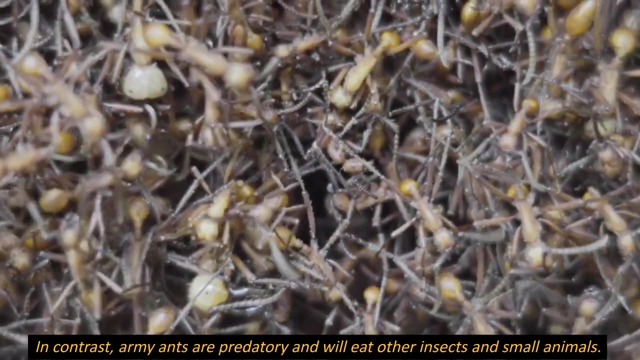 The type of food that ants eat will depend on their species and the location they inhabit. For example, some ants, such as leaf-cutter ants, feed on the fungus that they cultivate using leaves. In contrast, army ants are predatory and will eat other insects and small animals. 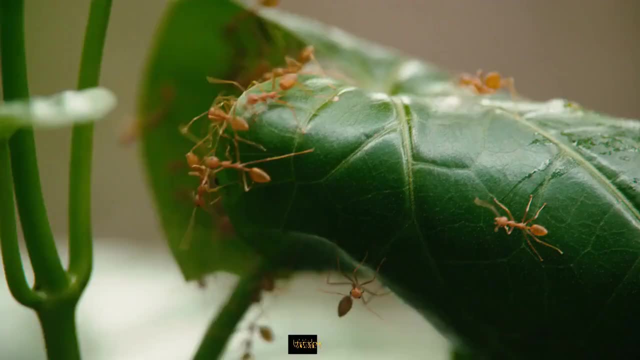 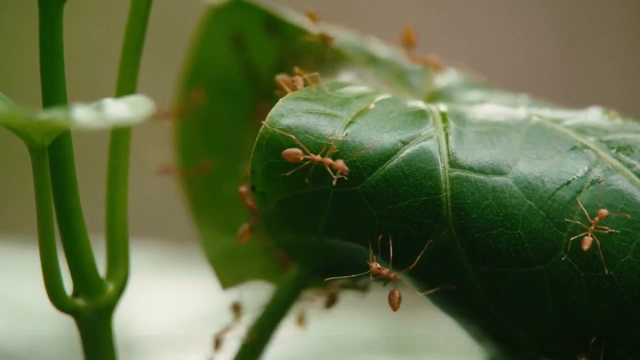 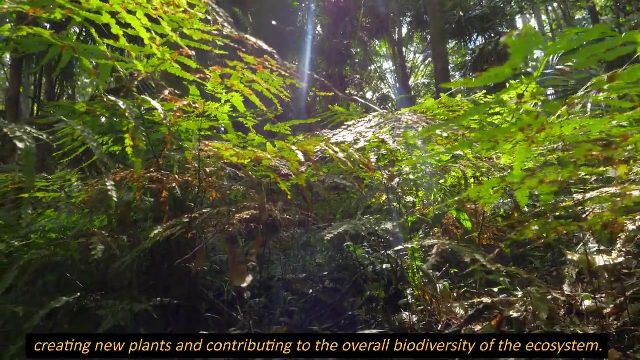 Ants Play a Critical Role in Food Web in seed dispersal. They carry seeds and fruits to their nests and feed on them, often discarding the remnants in their waste. These discarded seeds and fruits can germinate and grow, creating new plants and contributing to the overall biodiversity of the ecosystem. 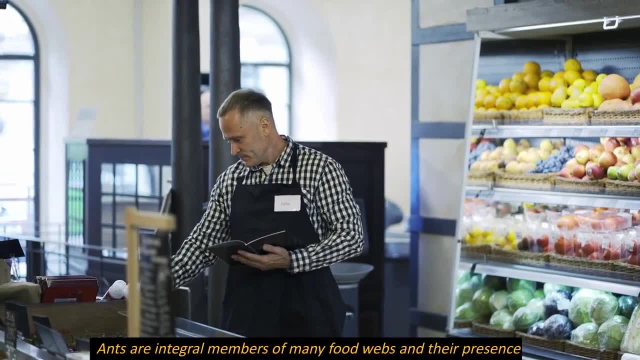 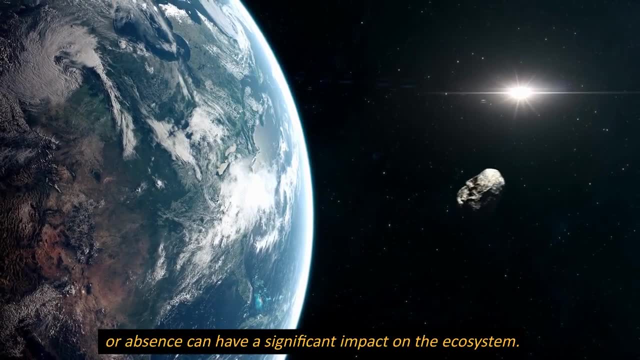 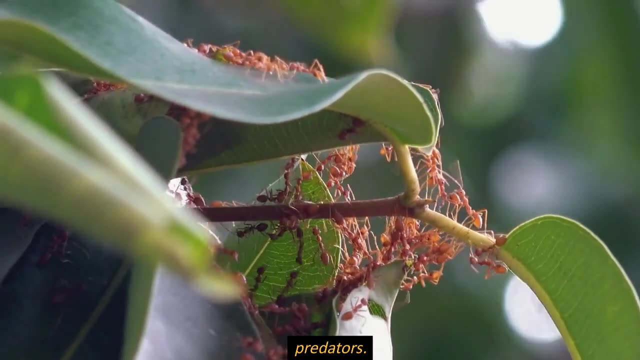 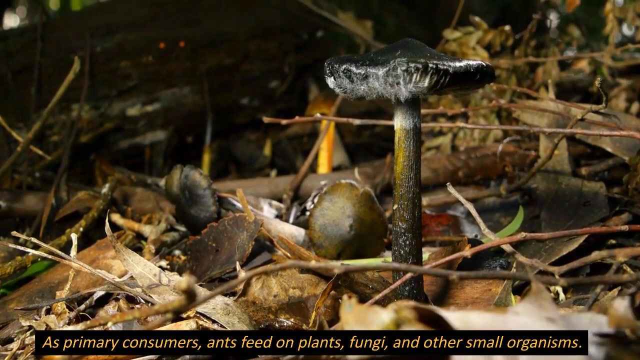 Role of Ants in Food Webs. Ants are integral members of many food webs and their presence or absence can have a significant impact on the ecosystem. Ants occupy various niches in food webs, from primary consumers to top predators. As primary consumers, ants feed on plants, fungi and other small organisms. They break down complex. 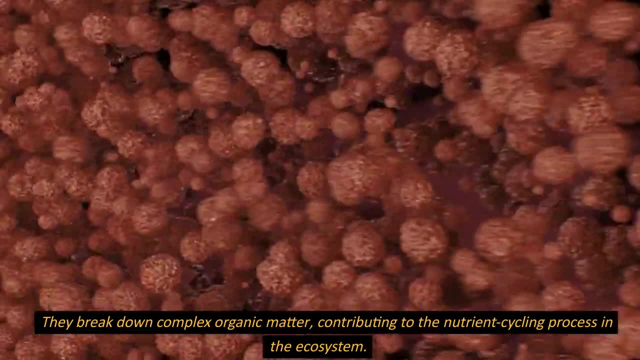 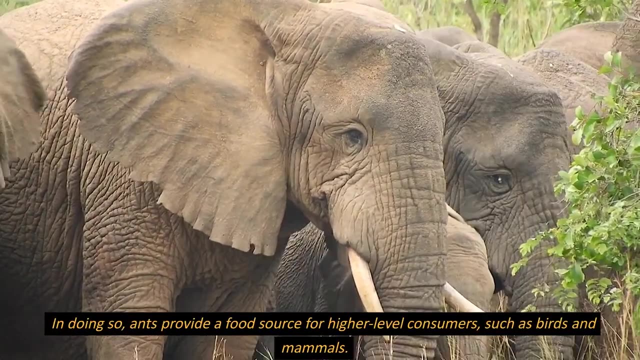 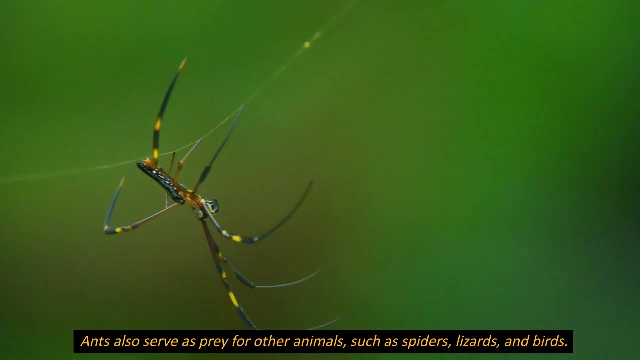 organic matter, contributing to the nutrient cycling process in the ecosystem. In doing so, ants provide a food source for higher-level consumers such as birds and mammals. Ants also serve as prey for other animals such as spiders, lizards and birds. They are an essential part of the diet of many. 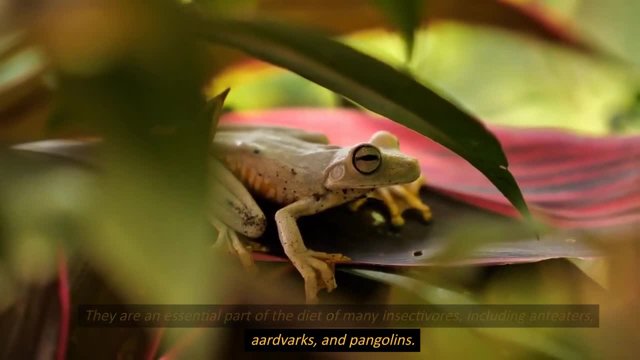 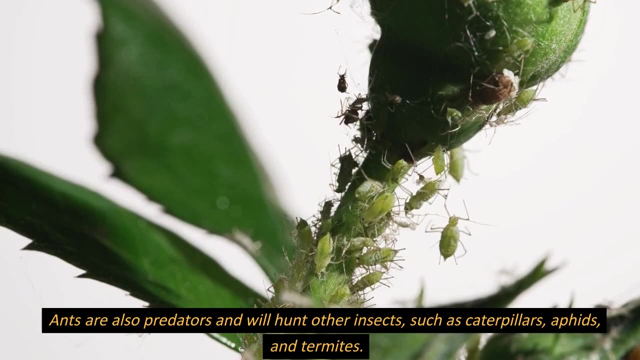 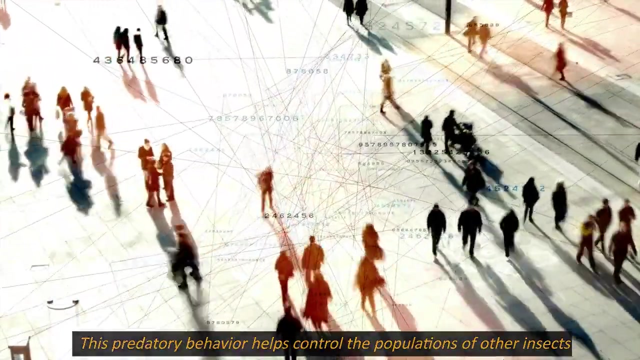 insectivores, including anteaters, aardvarks and pangolins. Ants are also predators and will hunt other insects such as caterpillars, aphids and termites. This predatory behavior helps control the populations of other insects and contributes to the overall balance of the 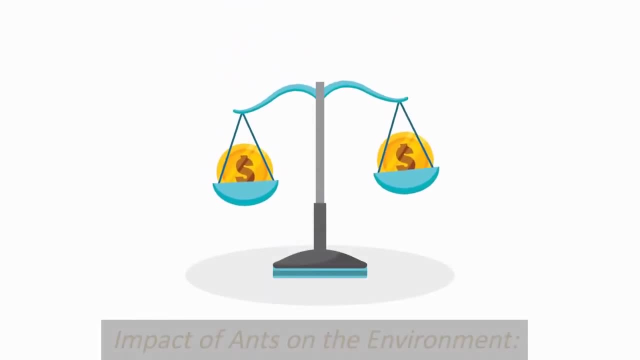 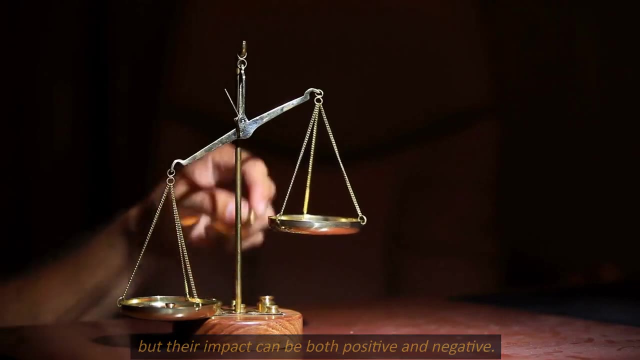 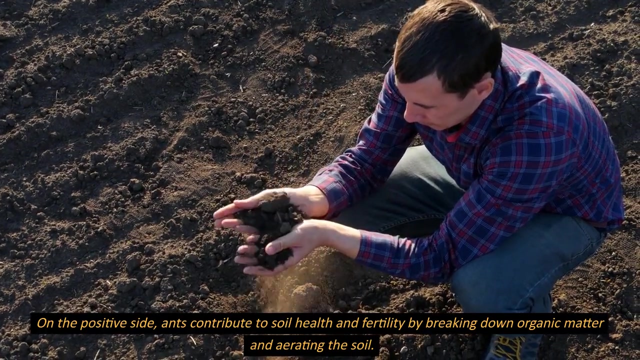 ecosystem: Impact of Ants on the Environment. Ants play an essential role in the environment, But their impact can be both positive and negative. On the positive side, ants contribute to soil health and fertility by breaking down organic matter and aerating the soil. Their foraging activities help distribute nutrients and 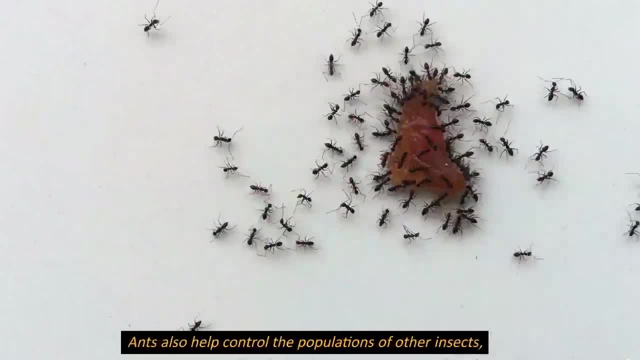 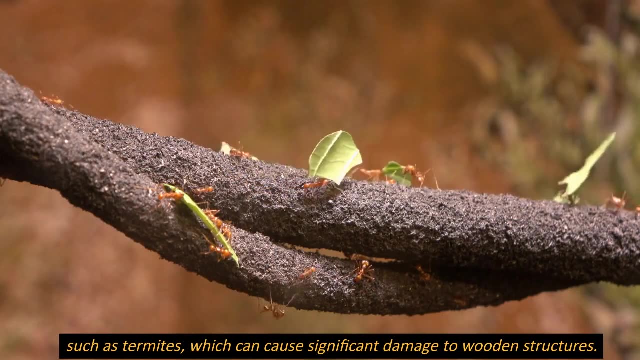 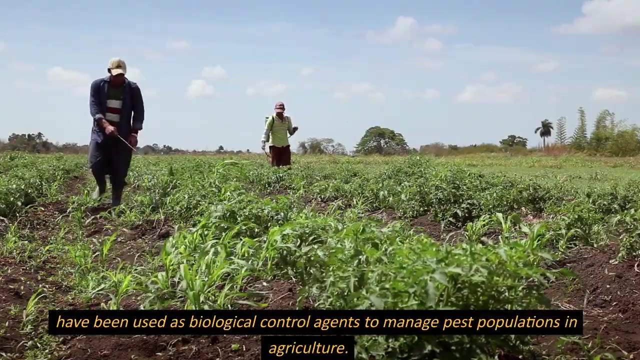 improve soil structure. Ants also help control the populations of other insects, such as termites, which can cause significant damage to wooden structures. Some species of ants, such as the Argentine ant, have been used as biological control agents to manage pest populations in. 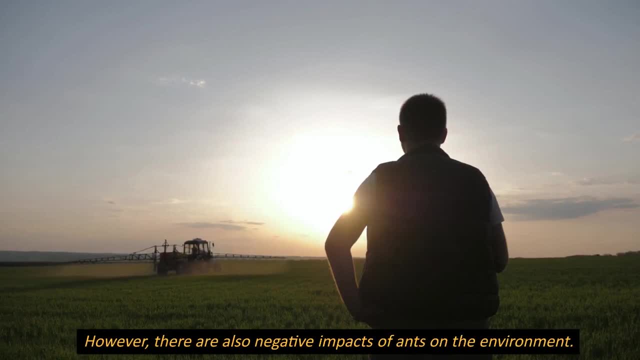 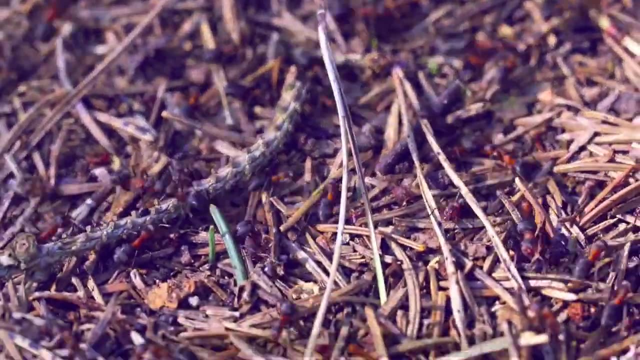 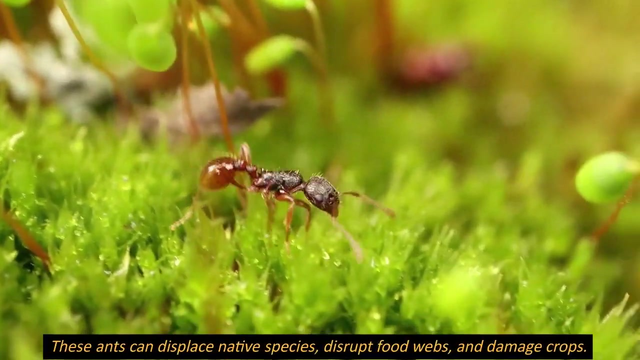 agriculture. However, there are also negative impacts of ants on the environment. Some species of ants, such as the Argentine ant, have been used as biological control agents to manage pest populations in agriculture. Ants are invasive and can cause significant ecological and economic damage. These ants can 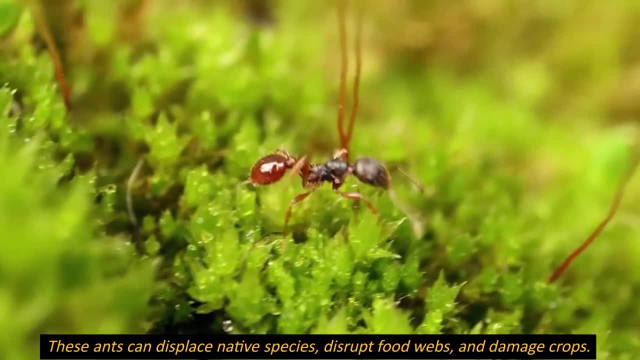 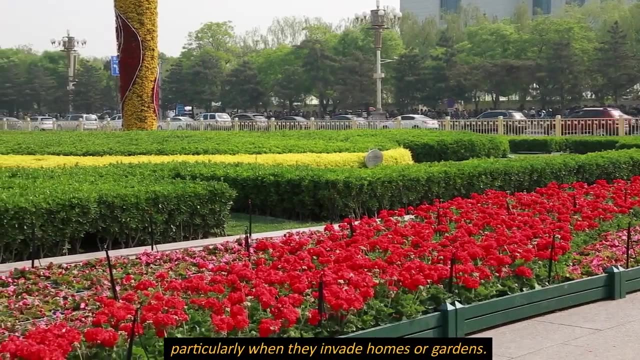 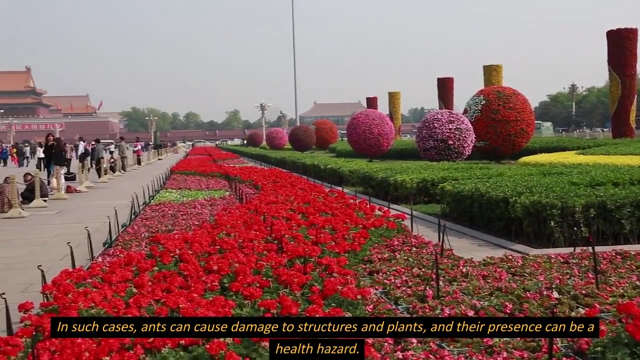 displace native species, disrupt food webs and damage crops. Ants can also be a nuisance to humans, particularly when they invade homes or gardens. In such cases, ants can cause damage to structures and plants, and their presence can be a health hazard. 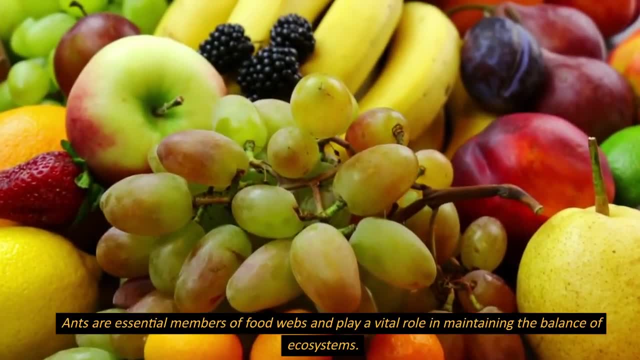 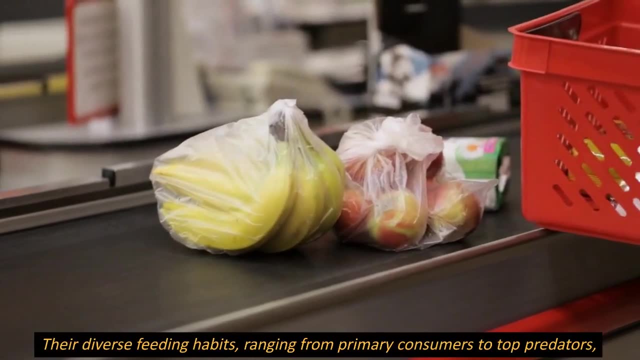 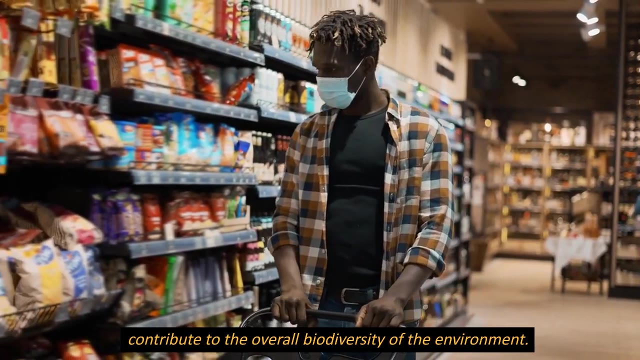 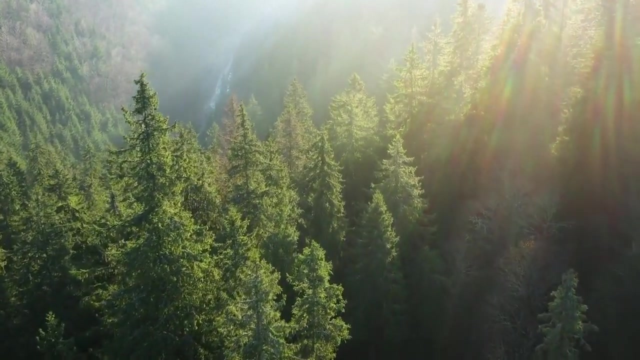 Ants are essential members of food webs and play a vital role in maintaining the balance of ecosystems. Their diverse feeding habits, ranging from primary consumers to top predators, contribute to the overall biodiversity of the environment. However, the impact of ants on the environment can be both positive and negative, and it is crucial to manage invasive species to 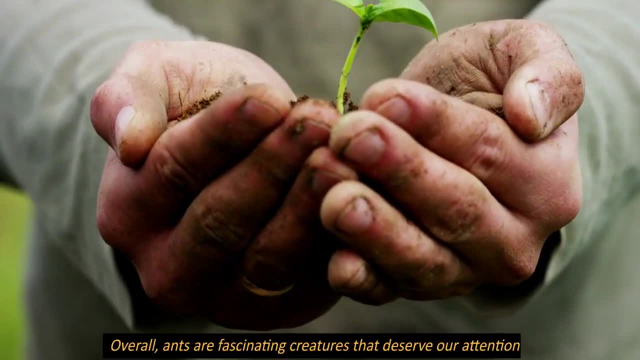 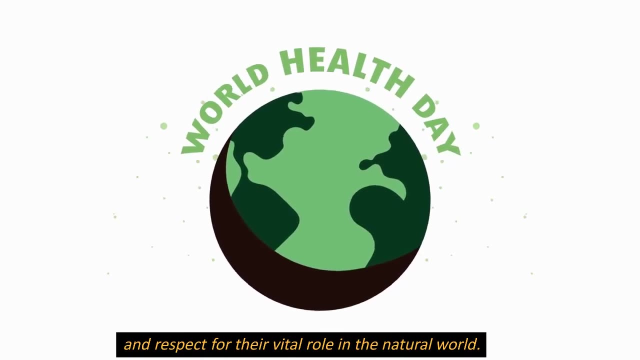 prevent damage to native ecosystems. Ants are also essential members of food webs and play a vital role in maintaining the balance of ecosystems. Ants are essential members of food webs and play a vital role in maintaining the balance of ecosystems Overall. ants are fascinating creatures that deserve our attention and respect for their vital role in the natural world. 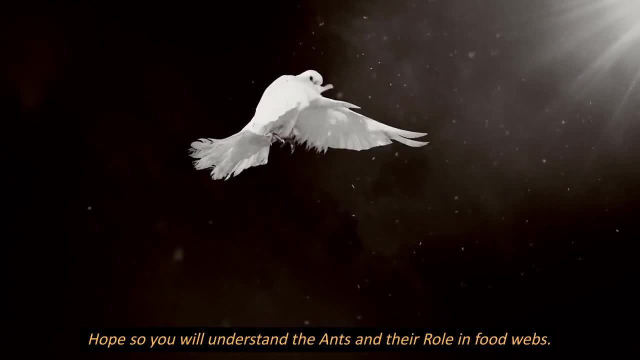 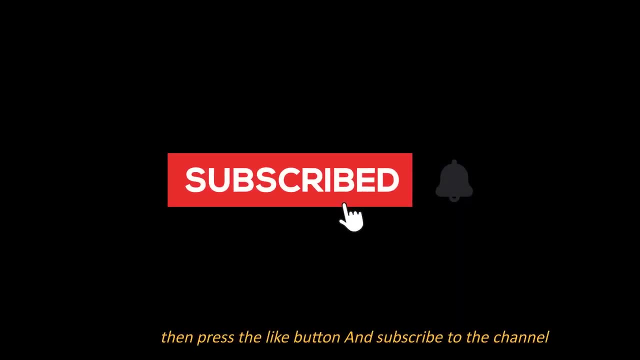 Hope so you will understand the ants and their role in food webs. Thanks for watching this content. if you like my content, Then press the like button and subscribe to the channel, And press the bell icon for upcoming videos. Thank you, Good bye.